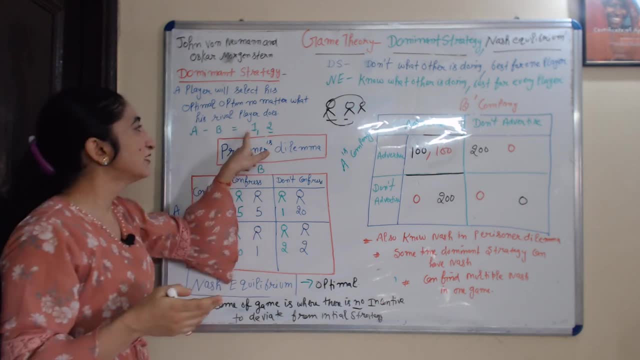 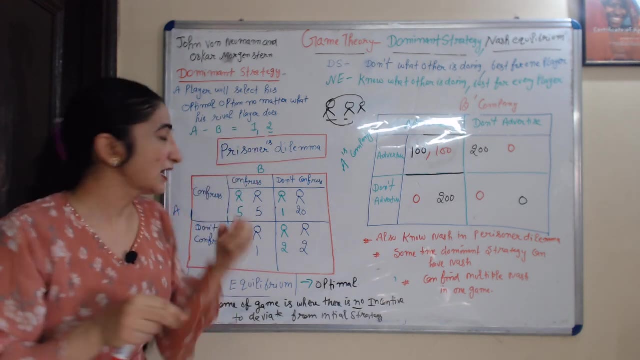 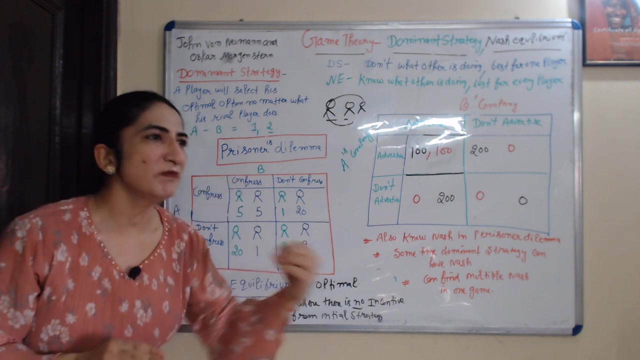 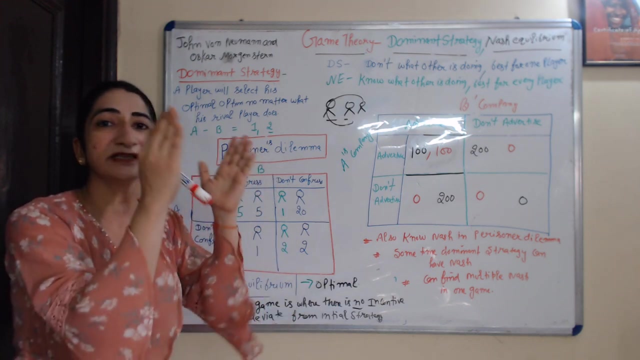 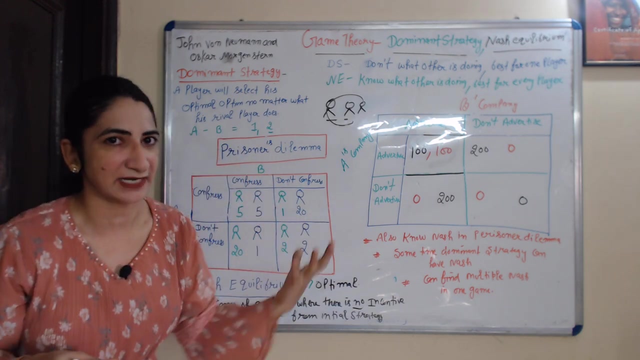 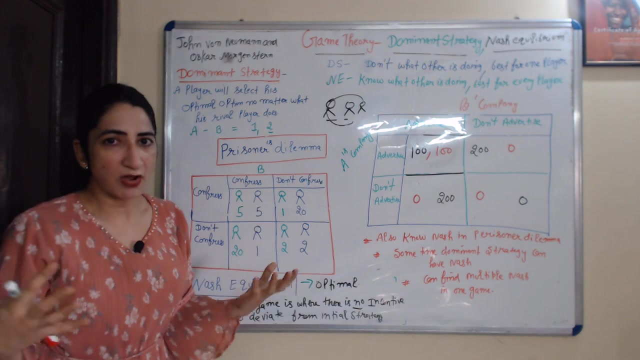 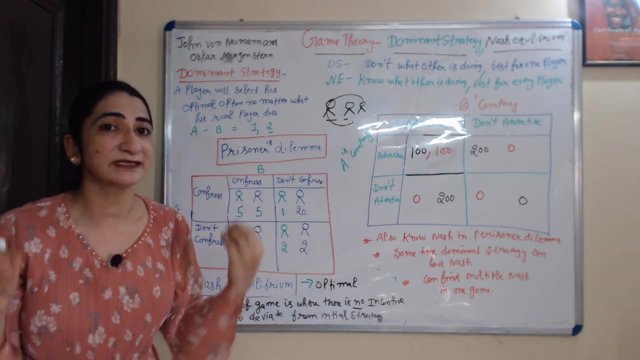 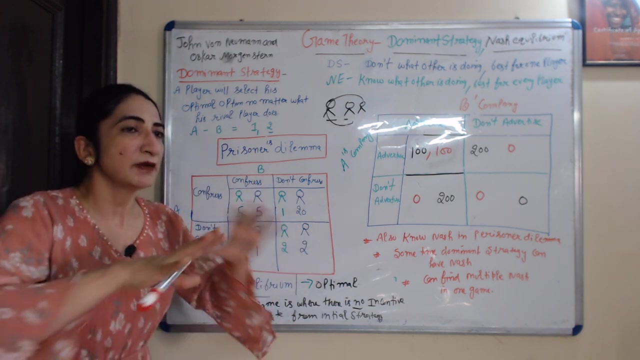 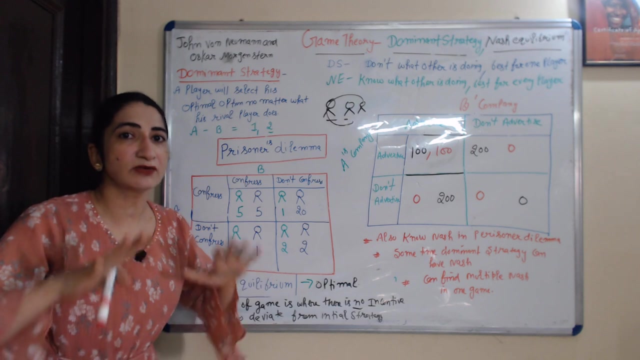 select his best possible option. Okay, for example, there is a game where a player will select his best possible option. Okay, for example, there is a game where a player will select his best possible option. Okay, for example, there is a game where a player will select his best possible option. 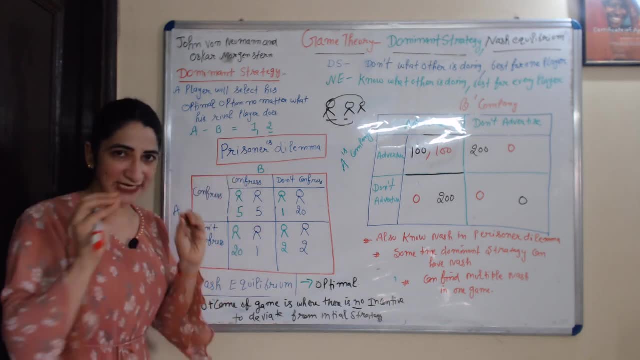 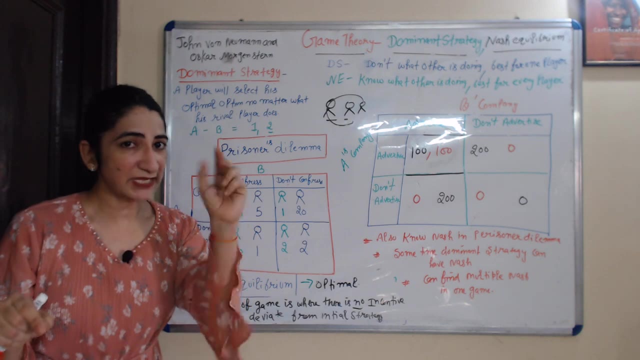 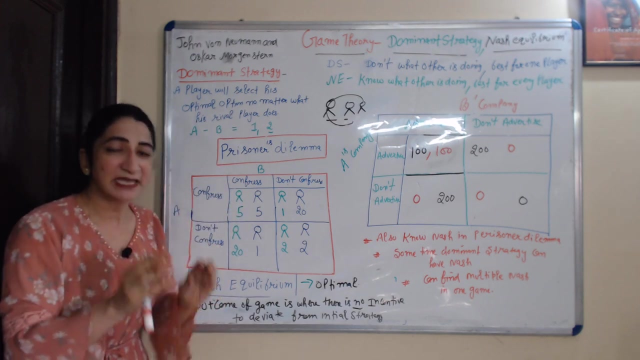 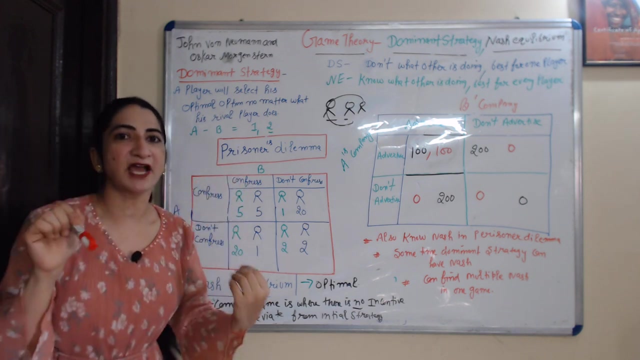 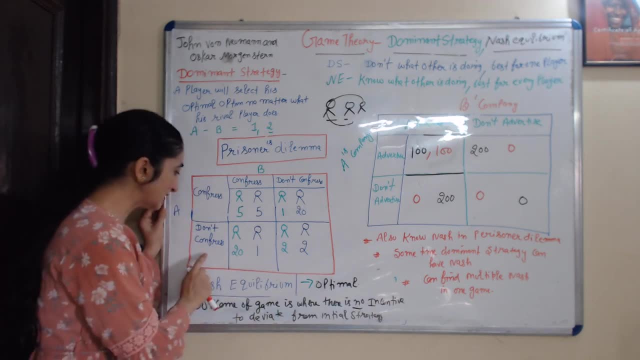 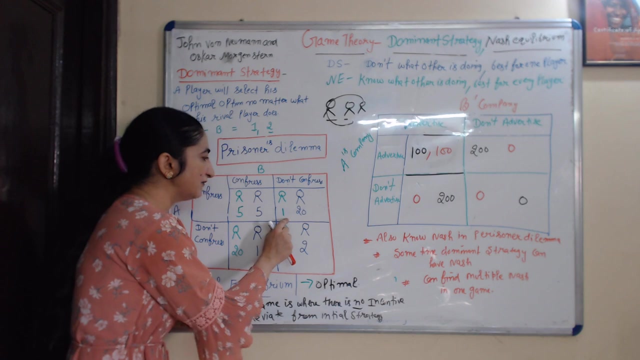 get two euro punishment. okay, if person a don't confess their crime but b confess, in this case, a will get 20 euro punishment and b will get only one euro punishment. if b don't confess their crime but a confess, in this case, a will get one year of punishment and b will get 20 euro punishment. and after considering or analyzing all this option, both select confession. after analyzing all these options, both select convention confession and okay b and a and b. both confess their crime in front of police and this is dominant strategy of both of them. this is best possible option for both of them. that's why this is called dominant strategy for them: confession. 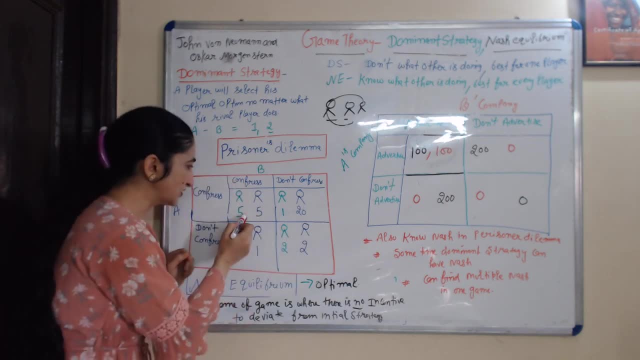 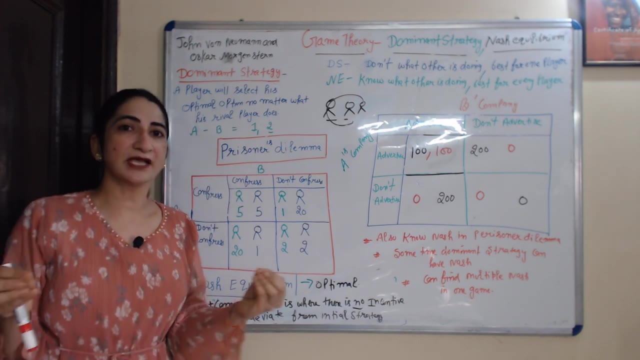 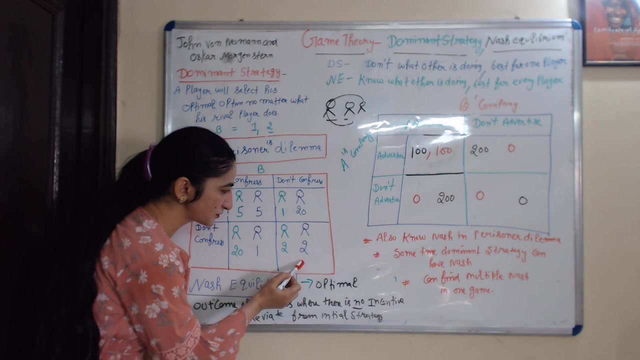 is dominant strategy for both of them. in case of confession, each will get five, five euro punishment. this is called best dominant strategy for both of them. now question is: how can we, how can we say that this is a best dominant strategy for both of them? they can select this option by not confessing. they will get only two year of punishment. that 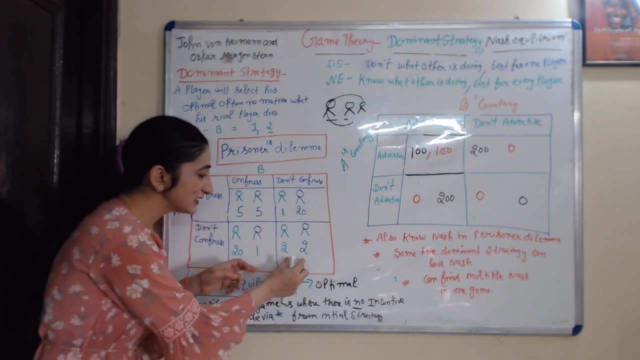 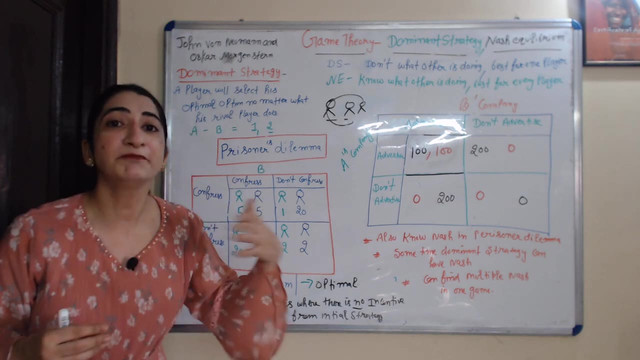 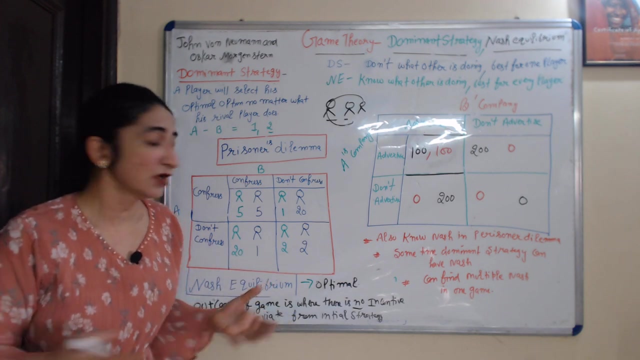 is very less from the five year of punishment. why did not they select this option? because this option is very risky. if a think i will not confess, then what happened if b confessed? in this case, a will get 20 euro punishment and b will get only one year of punishment. that is very unfair, oh. 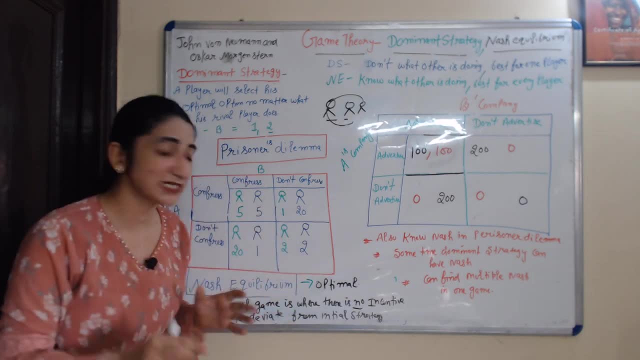 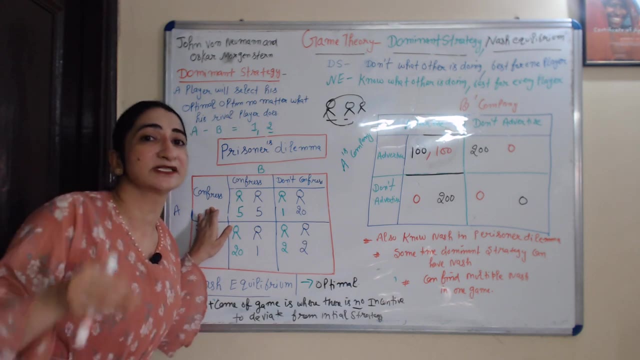 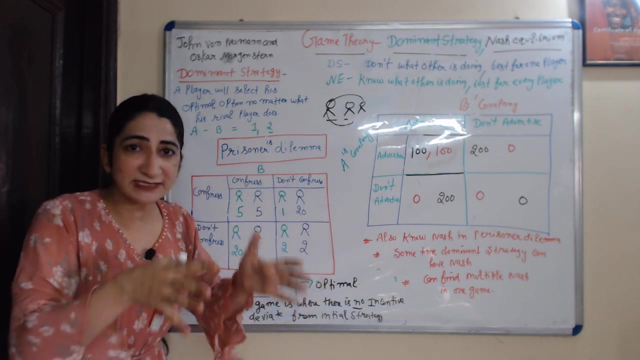 similar way. b will think so. this option is very risky. that's why they cannot select this option. after analyzing all this option, they will select confession. confession is best dominant strategy for both of them because when they select confession, they don't know about each other's strategy. because both are in separate lockup, they don't know about each other's strategy. 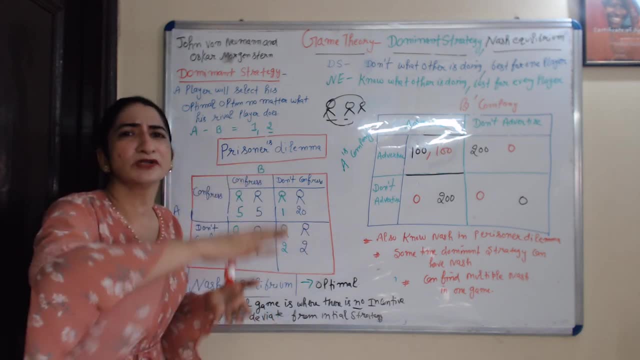 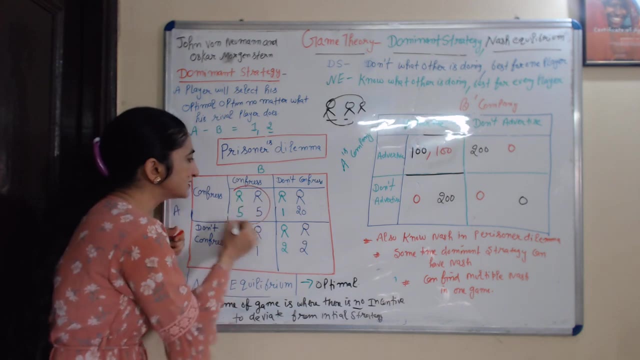 that's why they don't care about that. what other is going to select? they select confession because they think this is best strategy for them. okay, that's why this is called dominant strategy for both of them. okay, now nash equilibrium. what does mean by nash equilibrium? nash equilibrium in optimum outcome of game is where there is no incentive to deviate from its initial strategy. nash equilibrium we will get optimum output or we will get optimum outcome where- where there is no incentive to deviate from its initial strategy means in nash equilibrium we 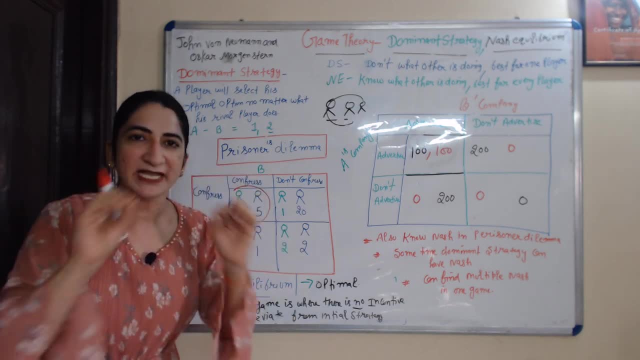 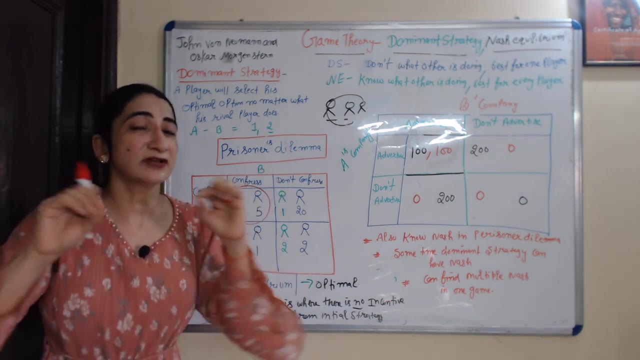 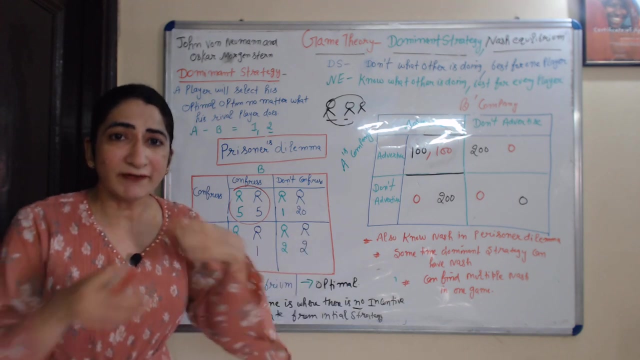 will get optimum point where none player cannot change their initial strategy. player cannot deviate from their initial strategy or we can say that player cannot move from their initial strategy. if player move from their initial strategy, they will get lows. we will understand nash equilibrium with a very simple example. okay, 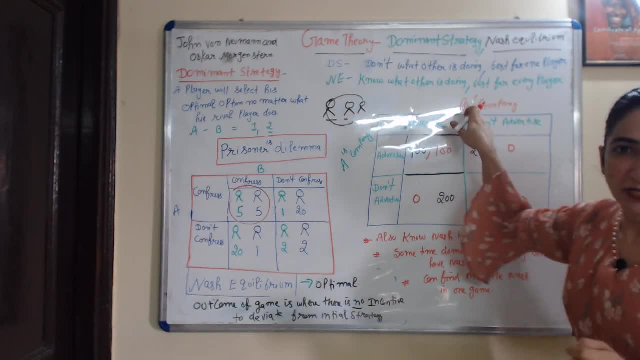 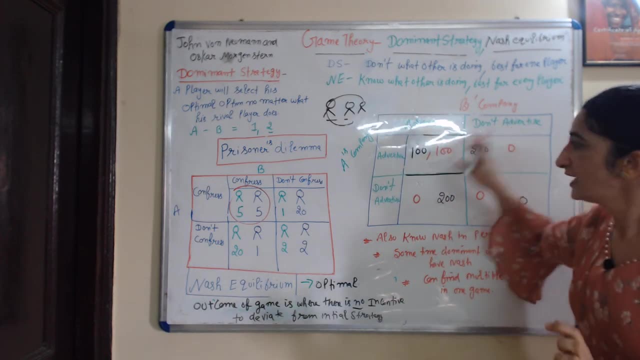 here there are two firm, a firm and b firm. okay, both have two uh option: either advertise their product or don't advertise their product. if both and b advertise, each will attract 100 customers. if both a and b form advertise, each will get a 100 customer. okay, if they both don't advertise, neither a advertise nor b advertise they will. 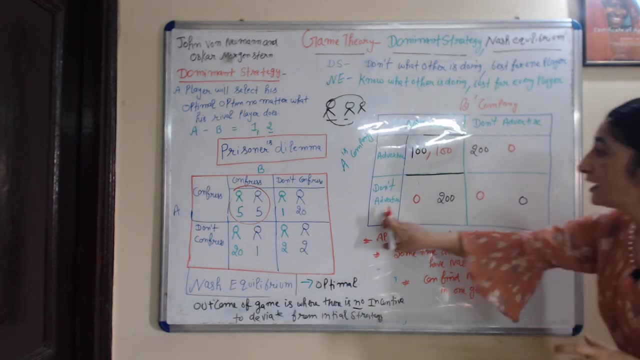 not attract any customer. they will attract zero, zero customer. if a don't advertise but b advertise, in this case, a will attract zero customer and b will attract 200 customers. okay, and b don't advertise but a advertise, in this case, a will attract 200 customer and b will attract zero. 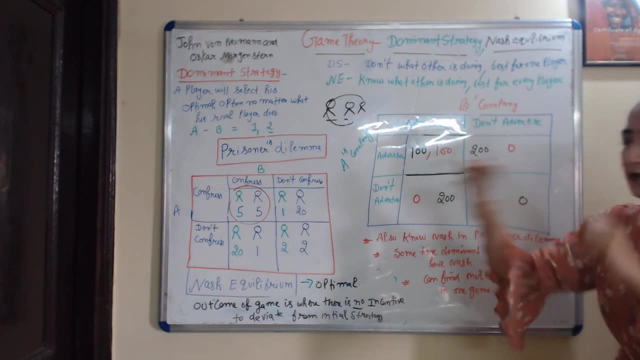 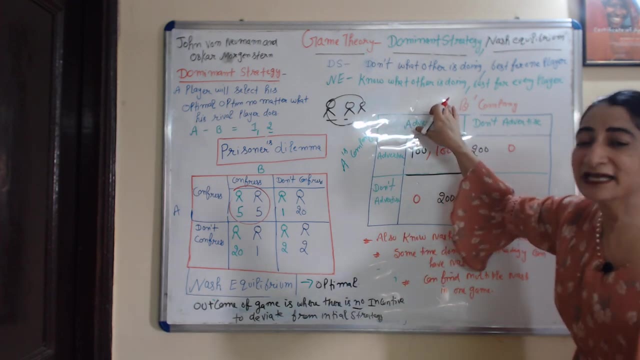 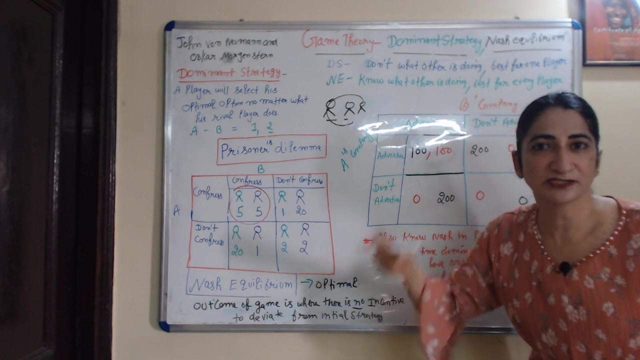 customer okay. then, for example, if b, if a know about b strategy, if a know about b strategy, b is going to advertise. in this case a will definitely advertise okay. if b, if a know about b strategy, b is going to advertise. in this case a definitely advertise okay, because because a can in. 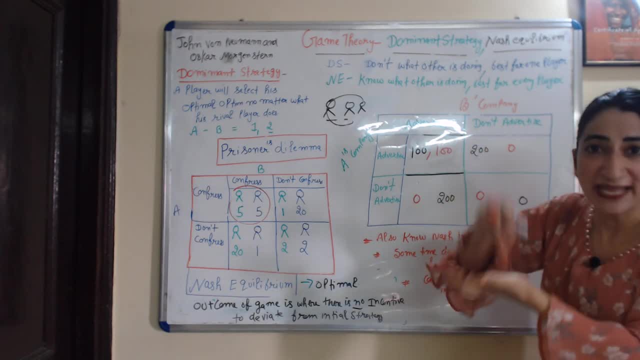 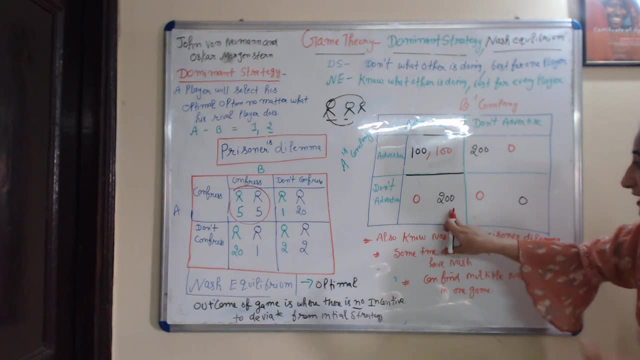 this case, a cannot change their initial strategy. if a change their strategy, they he will get low. you can see that if b is going to advertise, a will not advertise. in this case, b will attract 200 customer and a will attract zero customer. that's why a cannot change their initial strategy, because 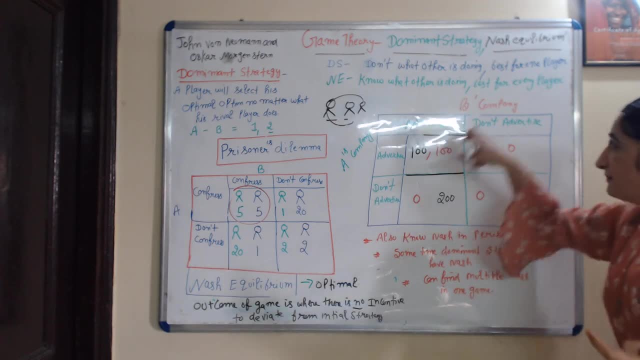 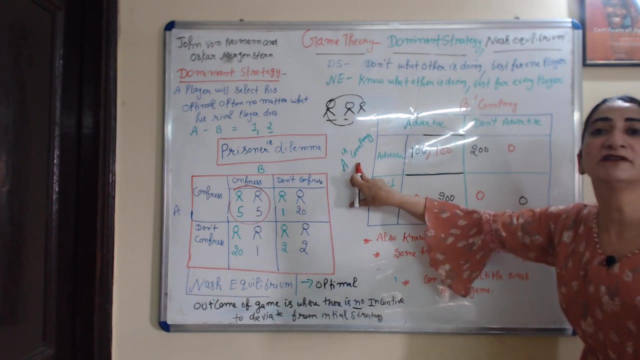 if we change their initial strategy, he is going to get a loss. similar in the case of b. if b know about a strategy he is going to advertise, then b definitely advertise. otherwise he will going to get a loss. okay, that's why a cannot change their initial strategy if a change their initial strategy. 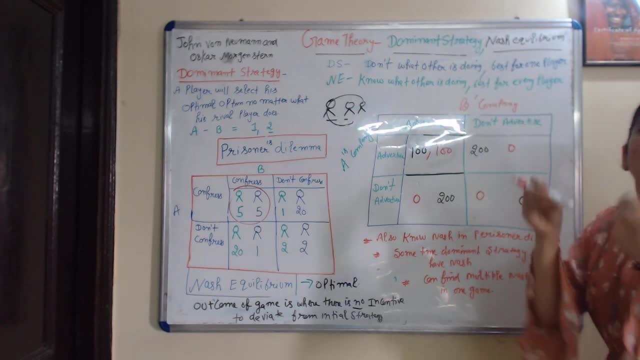 that's why, a after knowing each other strategy, both firm will advertise and they will get their dash equilibrium in this point. okay, this is best possible option for both of them. this is best possible option for both of them, a as well as b, and they can not deviate from their their at this. 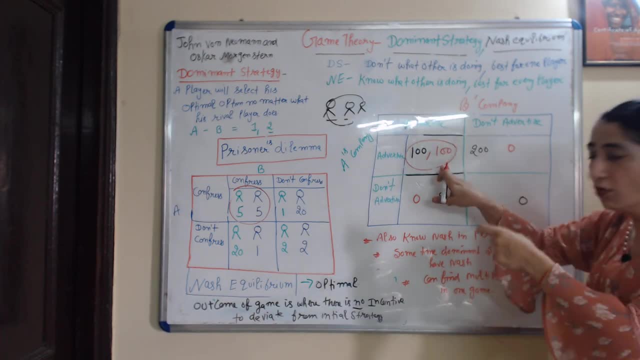 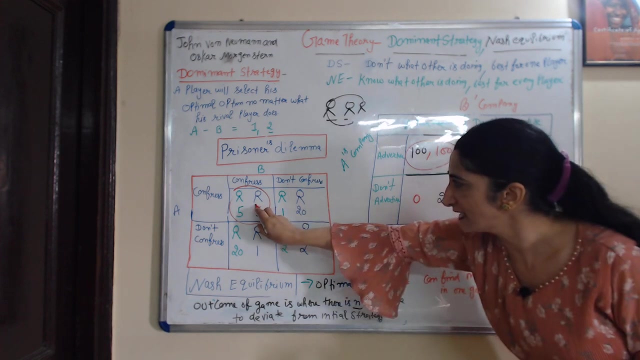 point. they cannot deviate from their this step. if they debate or move or change their, their strategy, they will. they will going to get a loss. okay, this is all about nash equilibrium most of the time. we strategy and a Nash equilibrium. okay, as we know, this is dominant strategy and 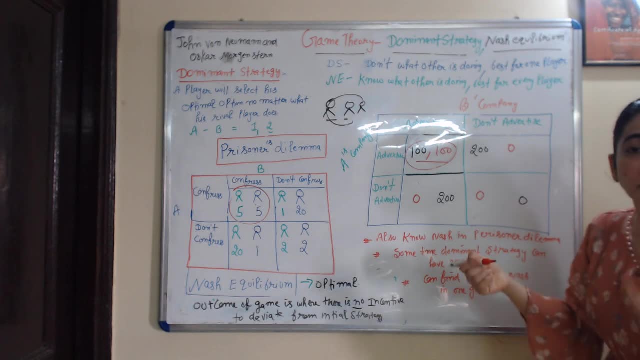 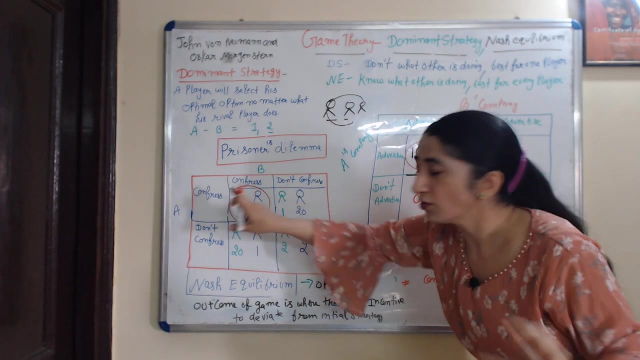 this is Nash equilibrium. okay, but we were confused between dominant strategy and Nash equilibrium. I will make you few differences though. in dominant strategy, we don't know what other is is doing. okay, we don't know about other person strategy, in this case, a and B are in separate lockup. okay, they don't know. 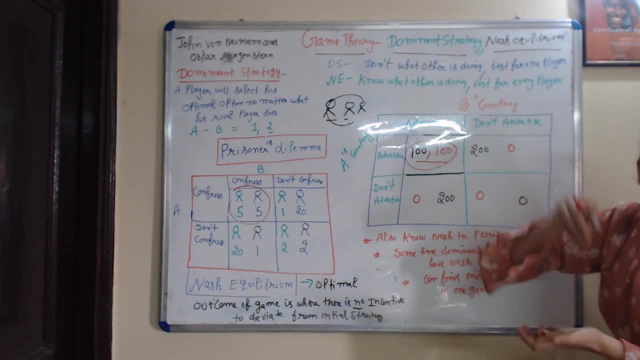 about each other strategy okay. but in Nash equilibrium we know about each other: strategy a, b, a. b a mean a know about B strategy and after knowing B strategy, a decide okay. similar being know about a strategy after knowing a strategy, B decide okay. but in dominant strategy we don't know about each other.